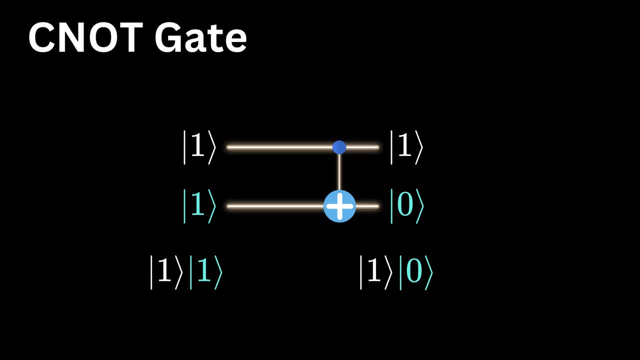 But don't let the tensor product intimidate you, as it can be simplified in common notation. we can represent it as one one and we can omit the tensor notation or even more simply, as one one in ket notation two qubits. unlike some powerful potential in 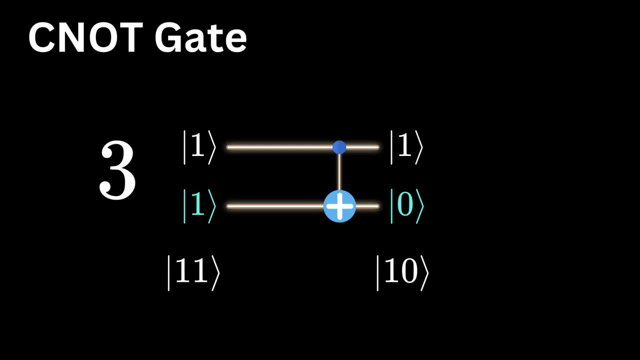 quantum computing with just two of them. we are able to encode numbers from zero up to three. four different states: one, one, a two qubit states in binary, which encodes the number three in our usual decimal system. we use this as our input for the quantum circuit and what comes out on the 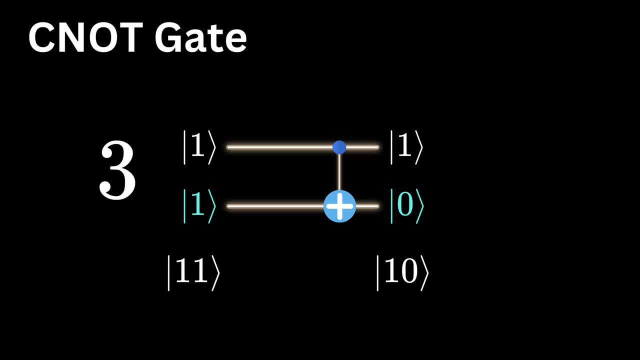 other side it's one zero, another two qubit state. in our everyday decimal system this translates to the number two. just like that we have mapped three to two. let's shake things up with the Hadamard twist towards CNOT gate. but what happens when we apply Hadamard gates on our 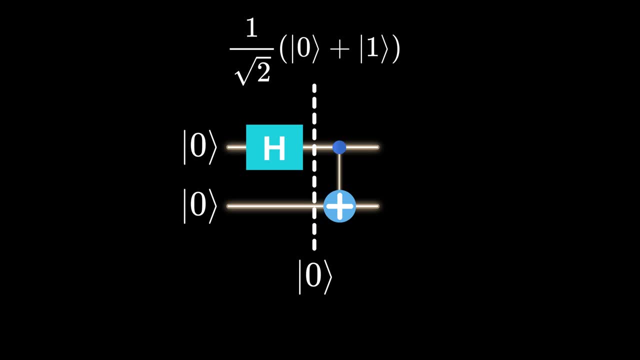 quantum circuit. we are able to vectorize it as our input and we are able to vectorize it as our. The Hadamard gate puts a control qubit into a superposition state, creating a balanced mixture of 0 and 1.. The state of the system so far is the superposition of 0 and 1 and the control qubit tensor product with the 0 and the target qubit. 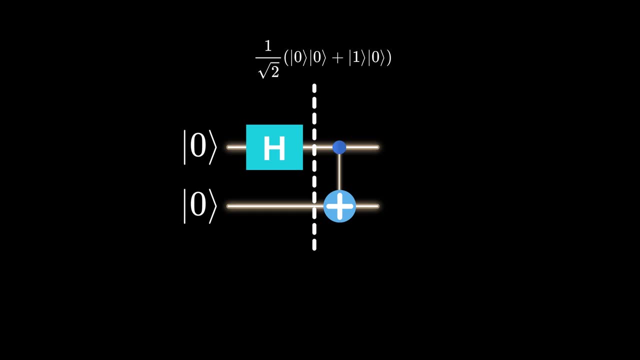 After doing a multiplication, the state of the system is the superposition of 0, 0 and 1, 0. Now let's send it through the CNOT gate. We know that CNOT is 0, 0.. CNOT is 0, 1.. 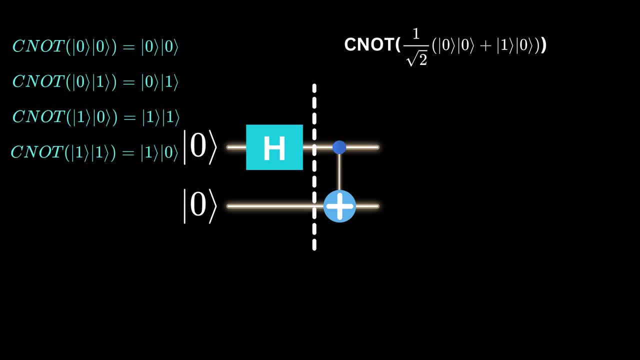 CNOT is 1, 1.. And CNOT is 1, 0.. So the CNOT is equal to CNOT plus CNOT, But remember that quantum gates are linear transformations, But CNOT is equal to 0, 0.. 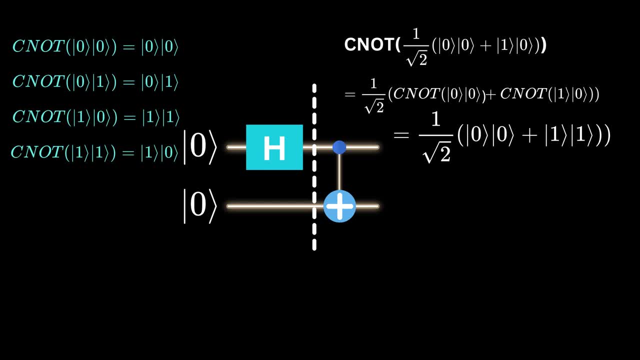 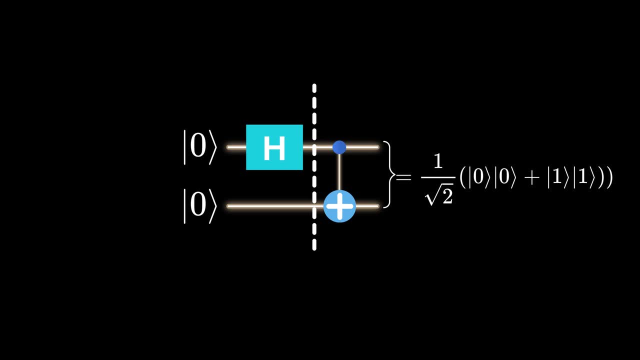 And CNOT is 0, 0.. CNOT is equal to 1, 1.. So the final state is 1 over square root of 2, 0, 0 plus 1, 1.. This combination results in a fascinating quantum behavior entanglement. 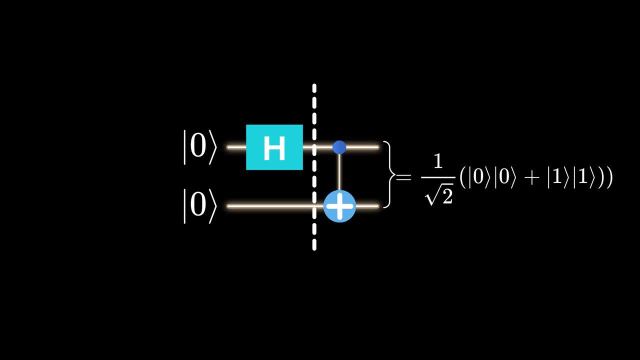 The state of our control and target qubits are now interconnected and cannot be separated. Even the great physicist Albert Einstein was confounded by this concept. He famously referred to entanglement as a spooky action at a distance, highlighted the mysterious and counterintuitive nature of quantum mechanics. 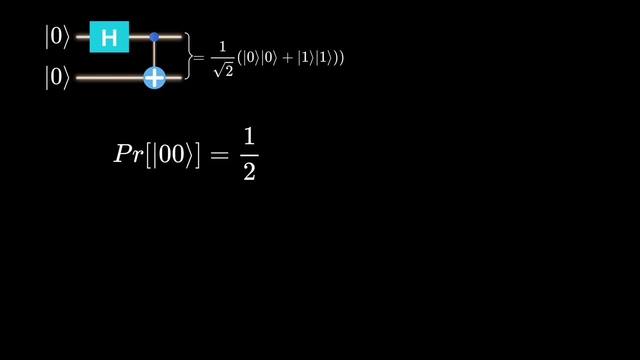 Entanglement is key to quantum computing, boosting computational power exponentially. In the case of an entangled pair of qubits, you will discover an interesting phenomenon: that the chance of both qubits being in the state 0, 0 or 1, 1 is exactly 50% each. 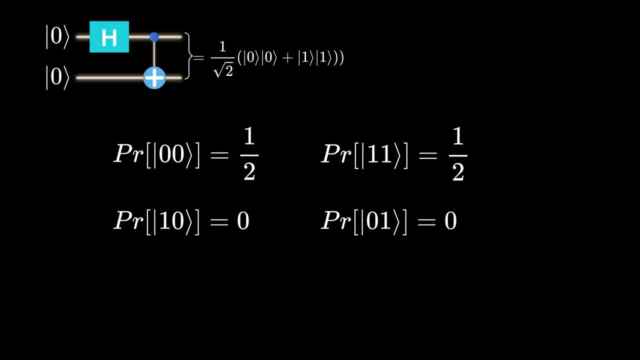 However, in the same scenario, the probability of finding them in the state 0, 1 or 1, 0 drops to 0, effectively making these states impossible. This counterintuitive outcome is part of the delightful mystery that makes quantum entanglement so captivating. 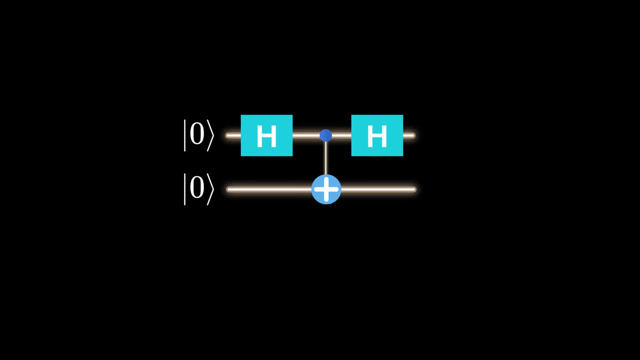 Imagine adding another Hadamard gate into our quantum mix, right after our CNOT gate. This adds another layer of complexity to our quantum circuit. What mysteries will this new addition unveil? Will it undo the entanglement? We have seen that the state of the system so far is superposition of 0, 0 and 1, 0. 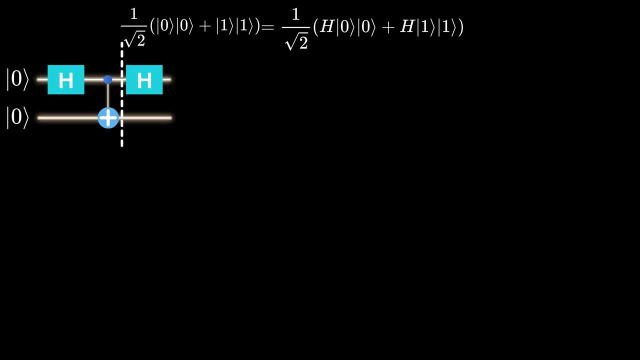 Now we apply Hadamard gate on the first qubit, which is a control qubit, But Hadamard gate on 0 is 1 over square root of 2, 0 plus 1.. And Hadamard gate on 1 is 1 over square root of 2, 0 minus 1.. 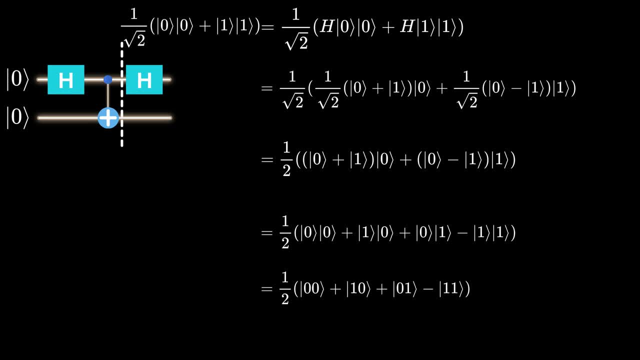 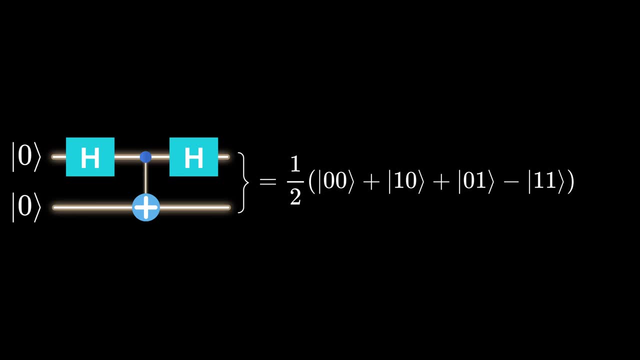 After simplification, we have superposition of 0, 0, 1, 0, 0, 1 and 1, 1, all with the same probability. The outcome is now a superposition of all possible outcomes. 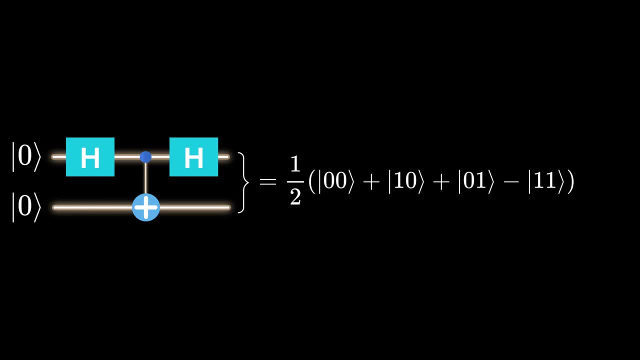 Yes, you heard it right. All possibilities are embraced at once. Instead of one definite state, we now have a dazzling array of potential outcomes. If we encode these two decimal representations, then we have a quantum function that maps 0 to the superposition of 0,, 1,, 2 and 3.. 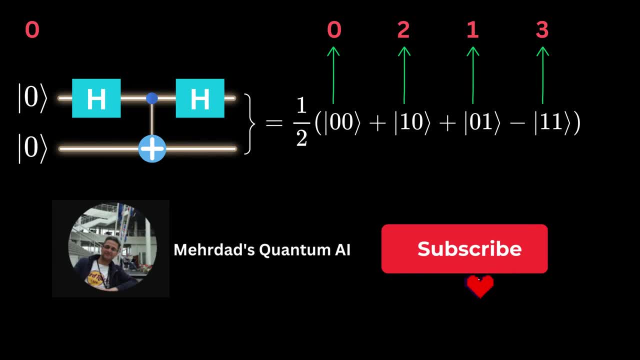 Thanks for watching today's video. If you enjoyed it, please like and subscribe, And don't forget to hit the bell icon for updates. Leave any comments or questions below. See you in the next video. Bye-bye.